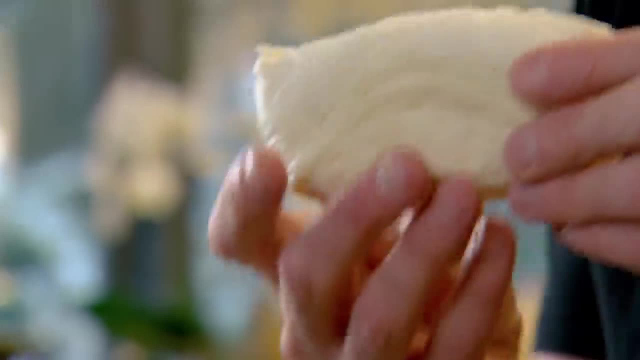 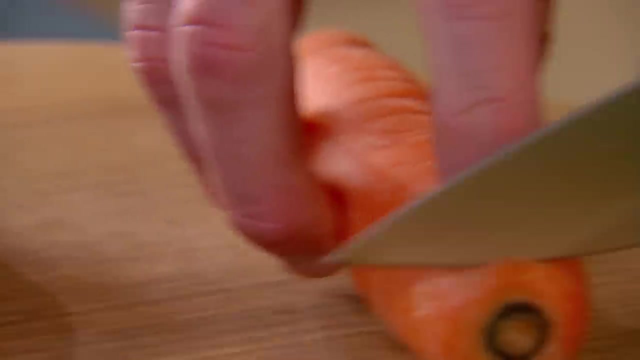 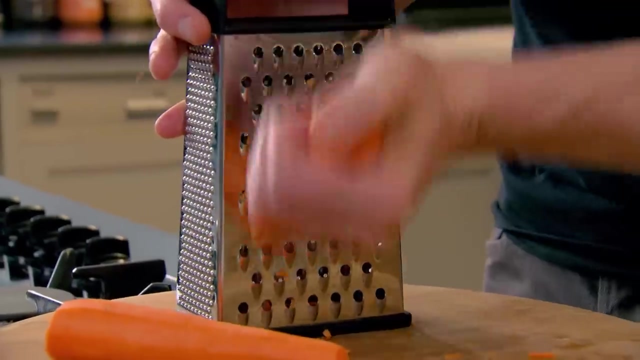 and cook long and slow for an hour and a half Now, halloumi cakes. There's something quite exciting about halloumi cheese. It's a very firm cheese and it fries brilliantly. Peel the carrots Great, Not too finely. 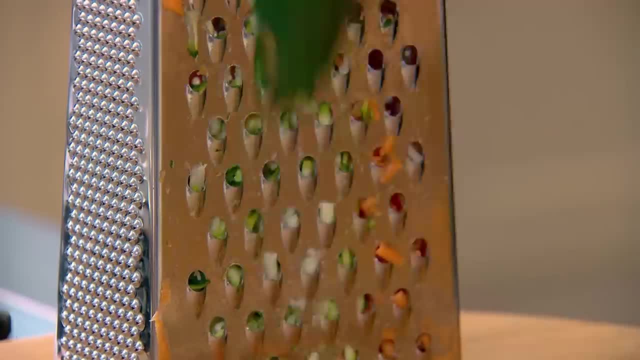 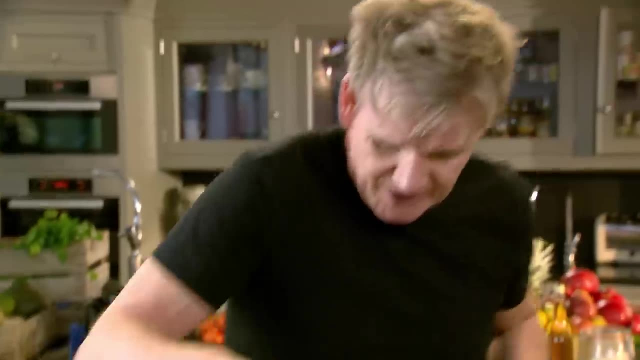 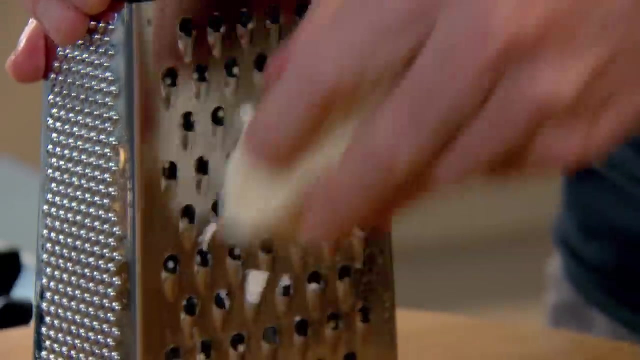 You want that nice texture. Next, courgette: The secret is keeping it all grated the same. Put that into a sieve. A sprinkling of salt will draw out liquid from the vegetables. Then grate the halloumi. Halloumi cheese doesn't look that tasty. 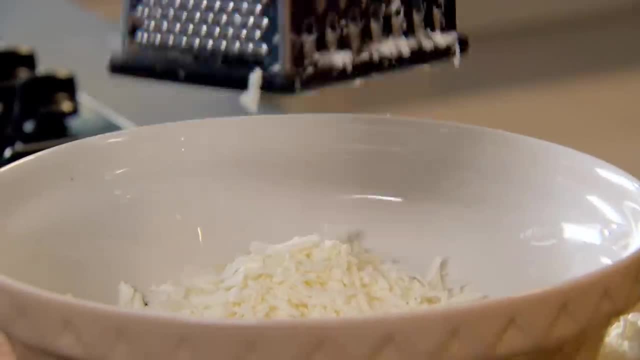 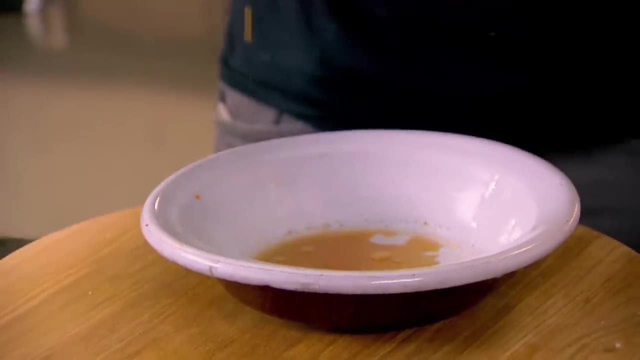 but once you've got colour on it in the pan, it's really, really delicious. Now really important to squeeze out the excess water from the veg. You'll see all that water that needs to come out of there. If you didn't do this, it'll make your little patties non-fryable. 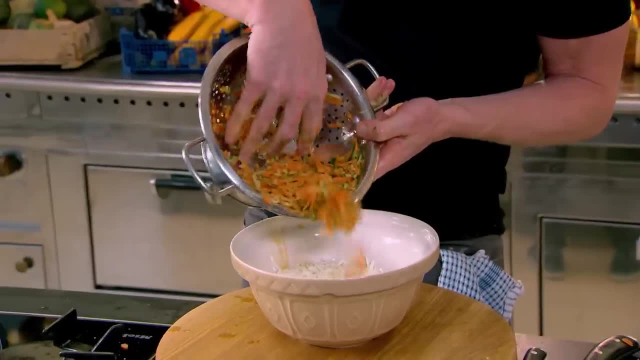 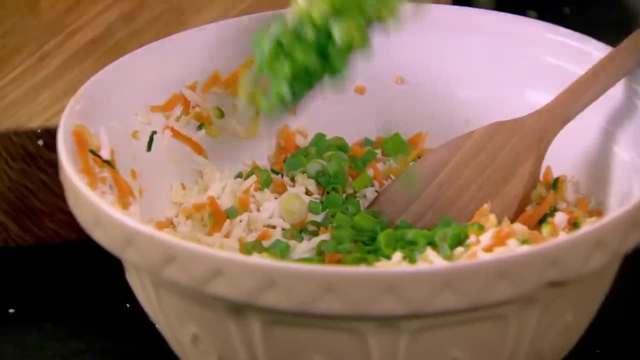 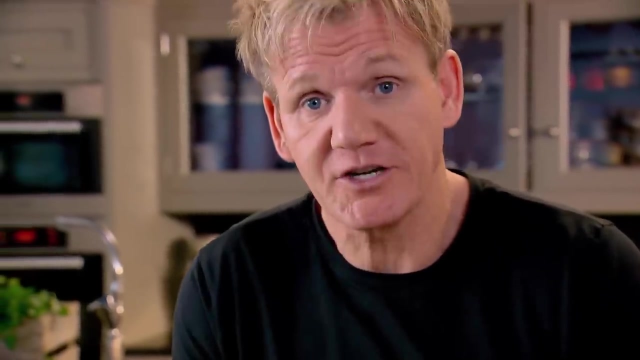 because the whole thing starts to separate And then mix in with the cheese: Spring onions, Chop up the whites and the greens. Now we're going to season that with some delicious fresh mint and fresh coriander. Whenever it's vegetarian, I like to put a combination of herbs in there. 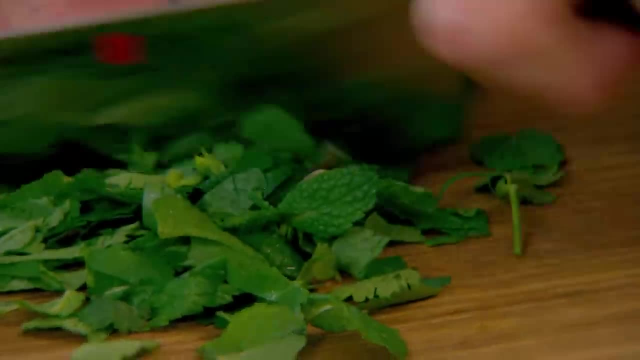 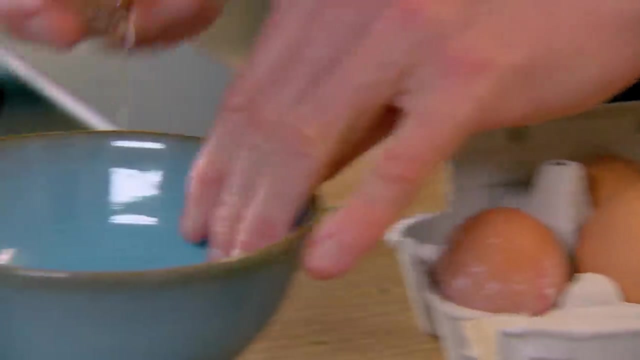 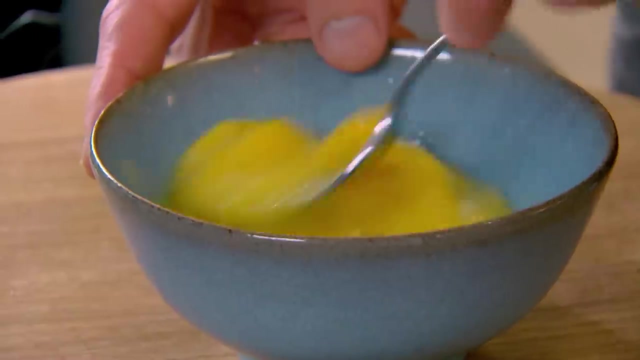 Tarragon and parsley, mint and coriander, basil and lemongrass. All delicious on their own, but in tandem their flavours play off each other. Next two eggs in. Give that a little mix. Add the eggs to the mixture. 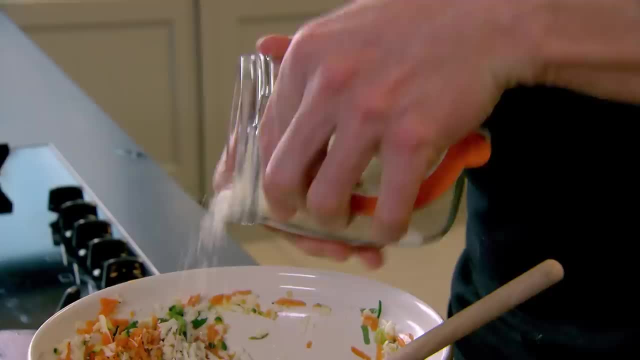 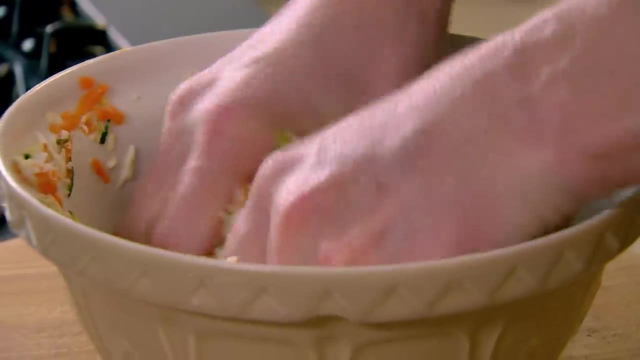 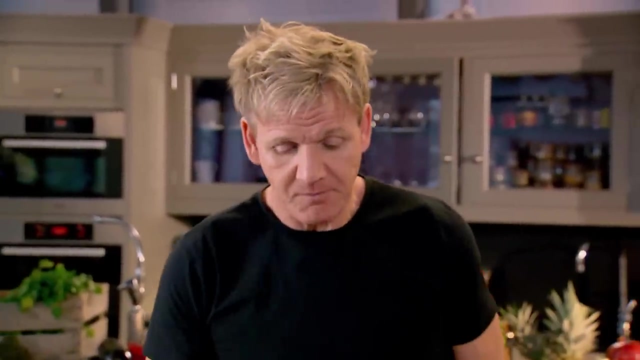 And then, finally, a couple of tablespoons of breadcrumbs. The breadcrumbs help dry out any excess moisture. Mix All the ingredients together Before you start shaping these, taste the mixture Mm. It's really important to identify the seasoning now, If you wait until you've cooked them. 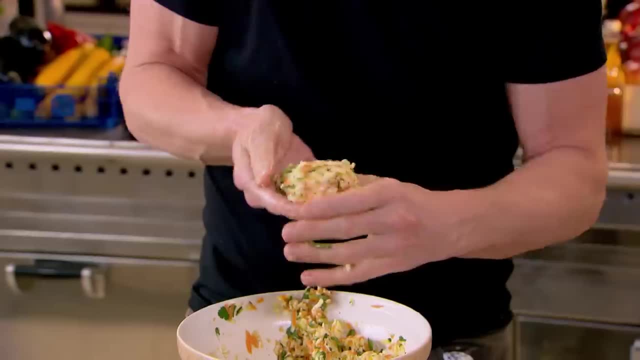 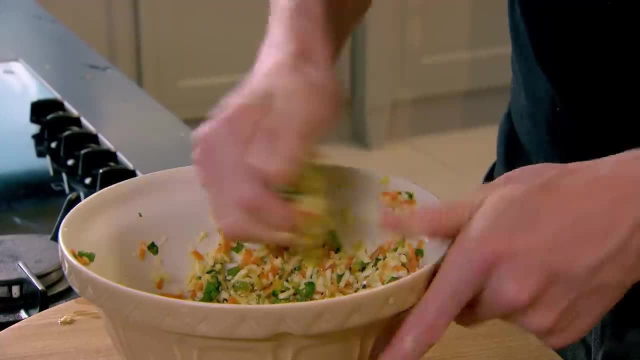 it'll be too late to adjust the seasoning. Roll them into a large golf ball, Shape them like a little mini burger. You could spice these up with some chilli in there if you haven't got fresh chilli Chilli flakes, And it's something that can be done up a day in advance. 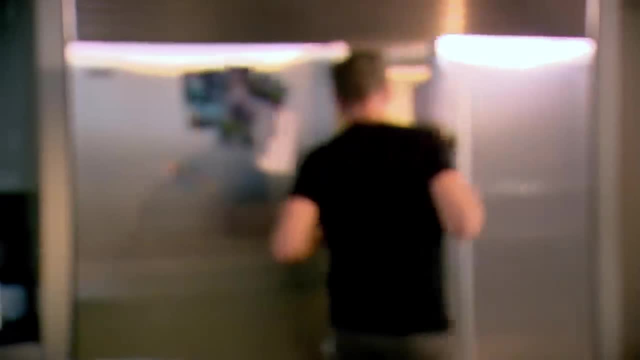 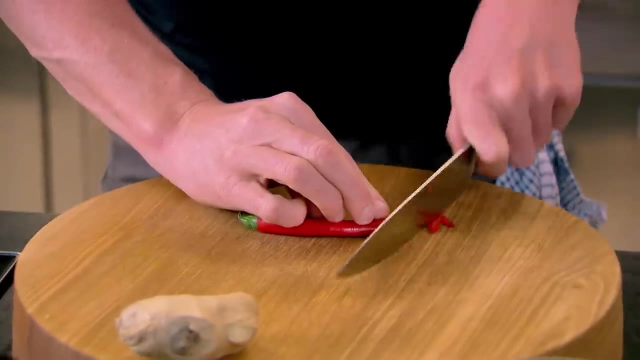 To get your cakes firm and ready for frying, put them into the fridge uncovered for 25 minutes. Pan on, Get that nice and hot. Whilst I'm waiting for that, I'll get the dressing ready. Slice the red chilli seeds and all, on an angle, into shards. 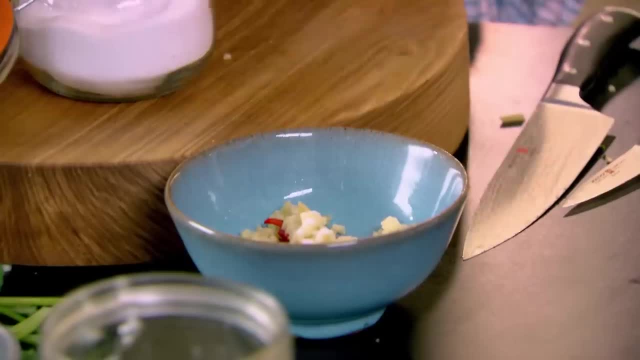 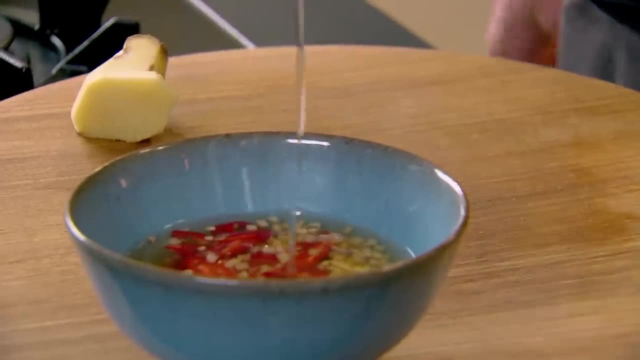 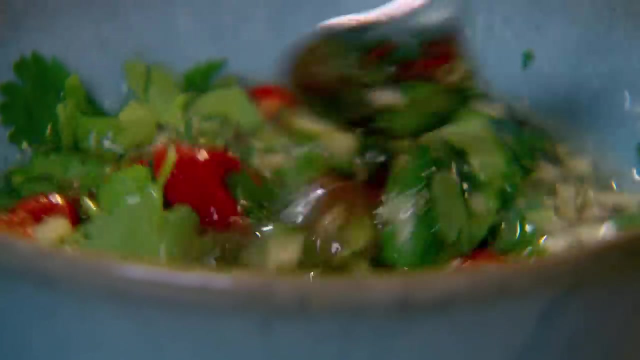 Then chop fresh ginger, Season with a sprinkle of sugar and salt, Add some rice wine vinegar, Add a couple of tablespoons of olive oil To finish off, some chopped coriander. MUSIC Got that sweet, sour, spicy flavour With my chilli dressing done. 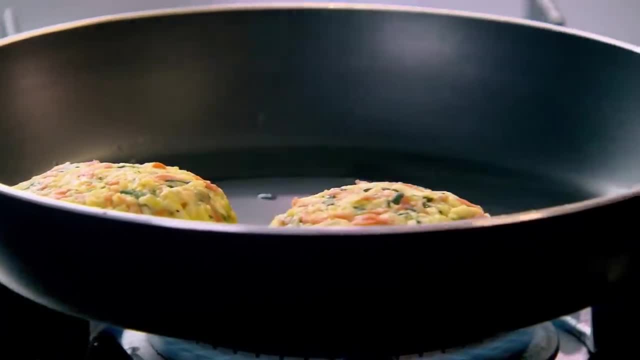 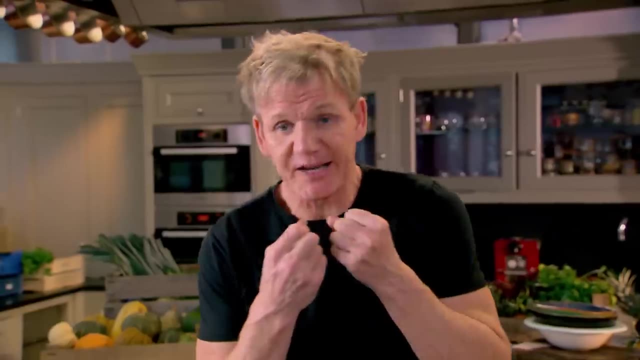 I can start frying off my halloumi cakes in a hot oiled pan. We get that nice crisp edge. You can already start to smell that sauteed halloumi with the courgettes and carrots Smells delicious. 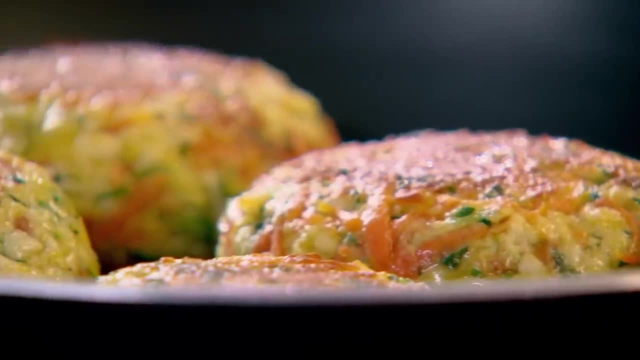 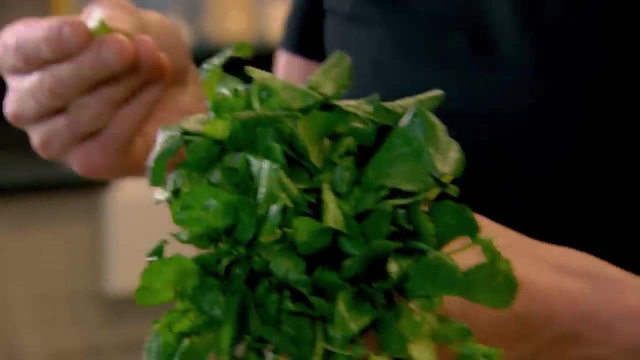 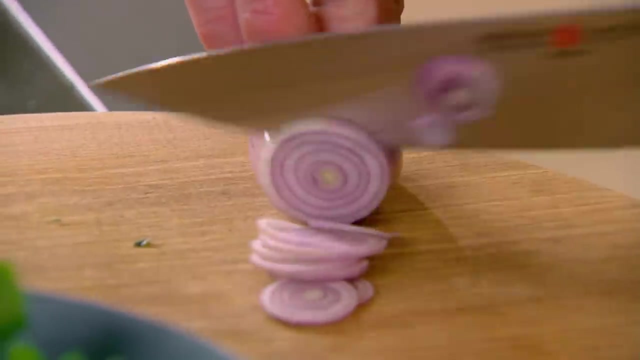 Really important to put a nice amount of colour on them. As my cakes sizzle away, I can finish off my roast tomato salad. One of my favourite leaves has to be watercress. Just cut off stalks, Shallot rings, Watercress and shallot go brilliantly well together. 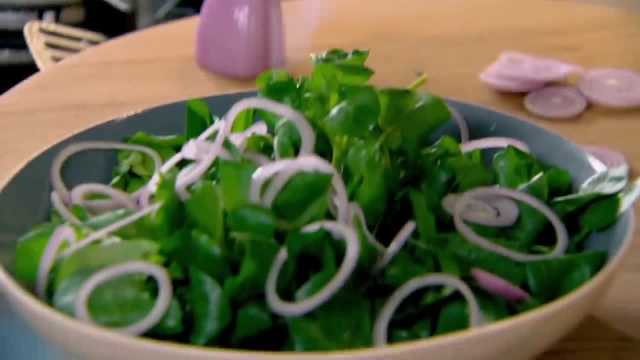 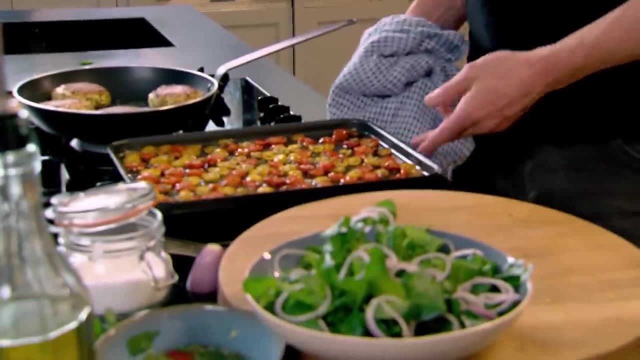 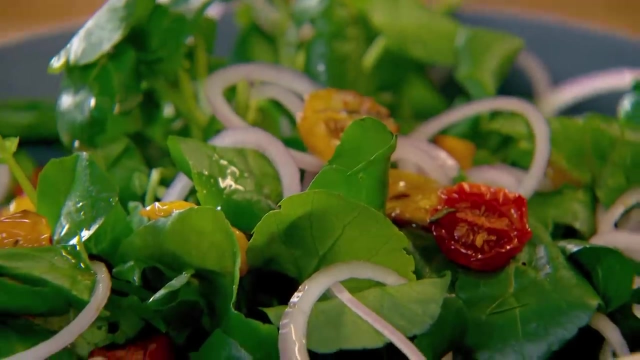 The shallot looks so dainty. when you open up these little ringlets, Don't forget to turn your cakes. Now tomatoes, Whatever you don't use. just jar them and put them in the fridge. Mmm, Just drop. Just drop those slow-cooked warm tomatoes over the watercress. 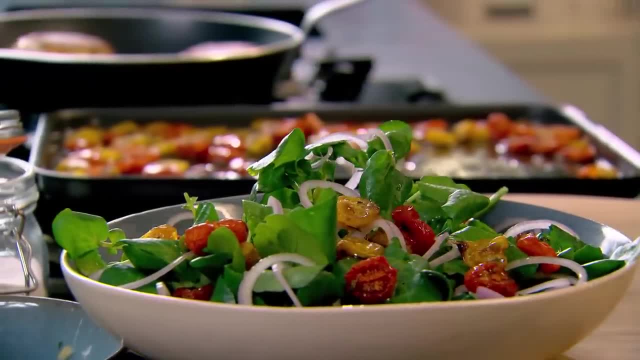 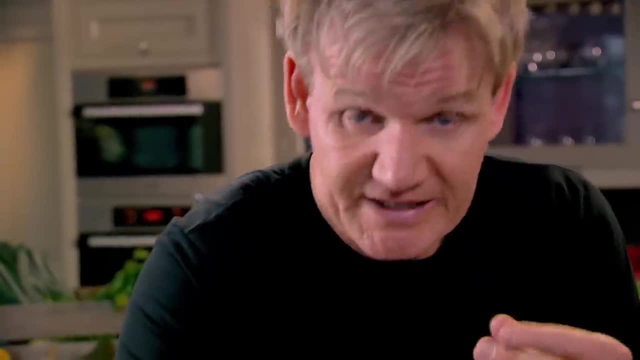 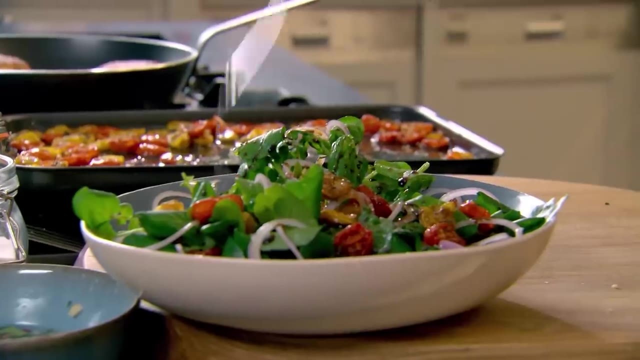 The sweetness is incredible, Absolutely delicious. A little drizzle of aged balsamic vinegar gives that tartness to the watercress. Watercress is naturally peppery, so it doesn't need any pepper, Just a little touch of salt and then a light sprinkling of extra virgin olive oil. 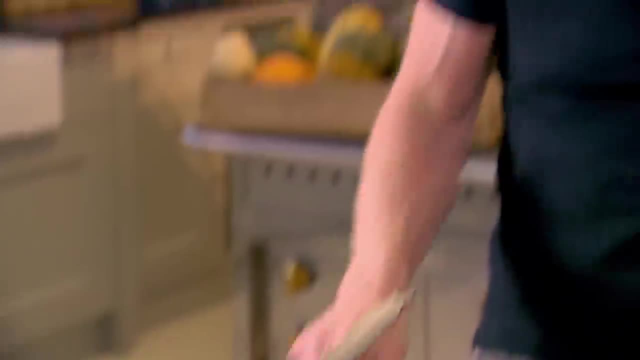 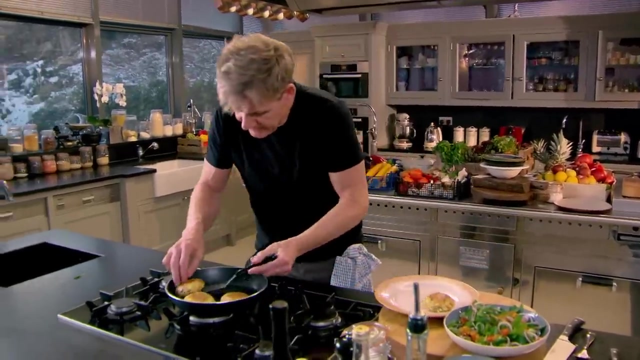 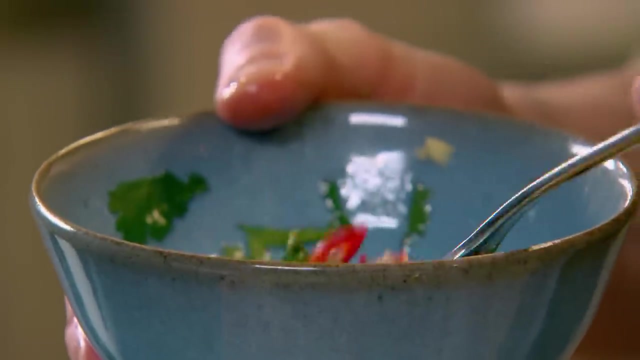 After five minutes on a medium heat, my halloumi cakes are ready. So important, So important to have taken out that water- You can see it doesn't disintegrate- And then just get your dressing, Take a spoon of it and then tilt it to the side. 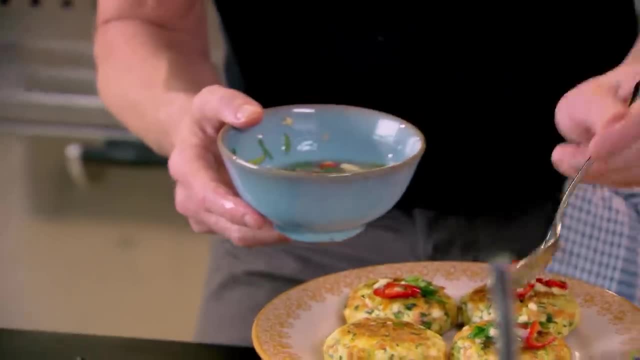 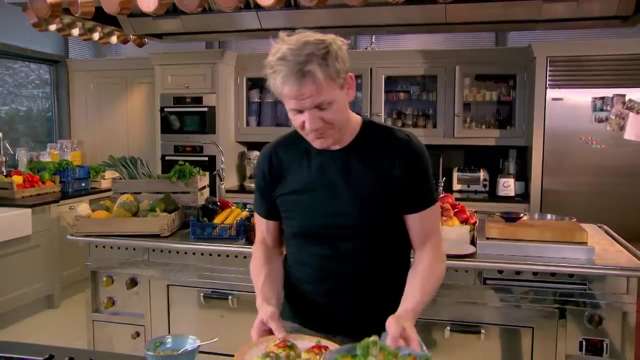 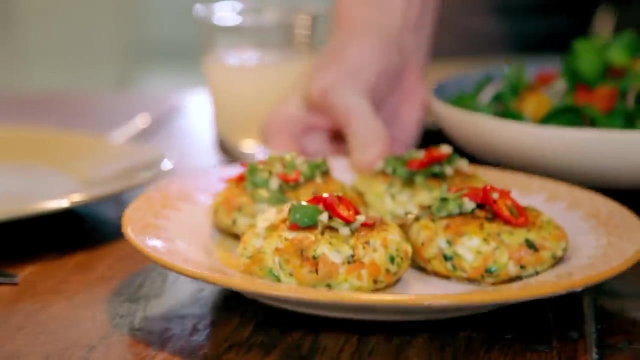 because I want the garnish, I don't want the juice. If that does not turn you on to become a vegetarian for the night, I honestly don't know what will. Delicious My crispy golden halloumi, courgette and herb cakes. 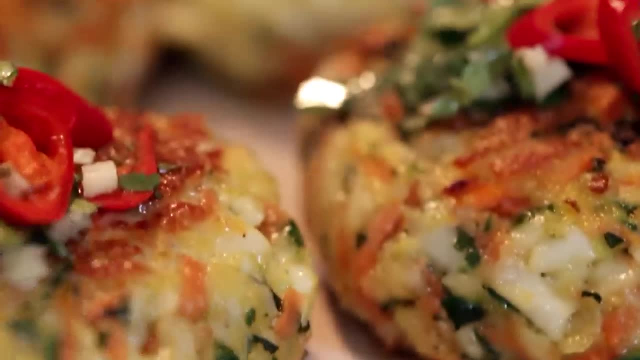 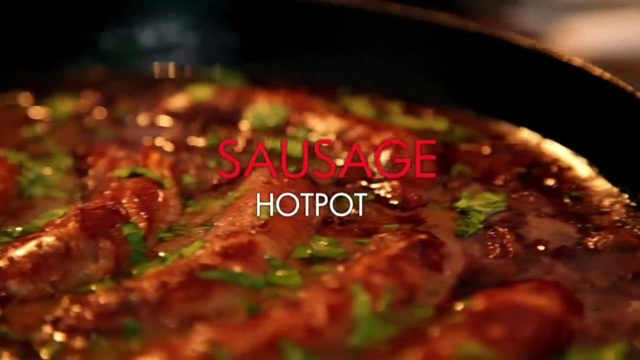 with a sumptuous roast tomato and watercress salad. all of the flavour with none of the meat. My ultimate comfort food dinner is a stunning sausage hot pot which will serve with a gorgeous potato and beetroot gratin. Now, I love hot pot. 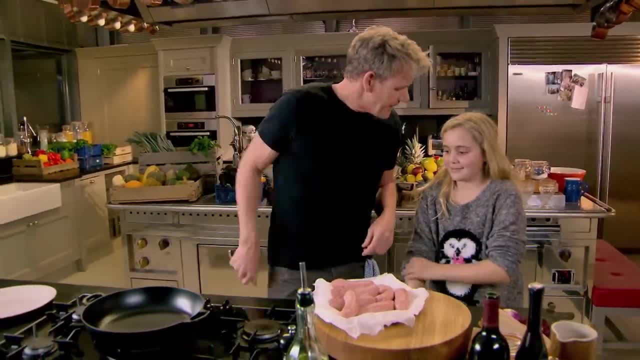 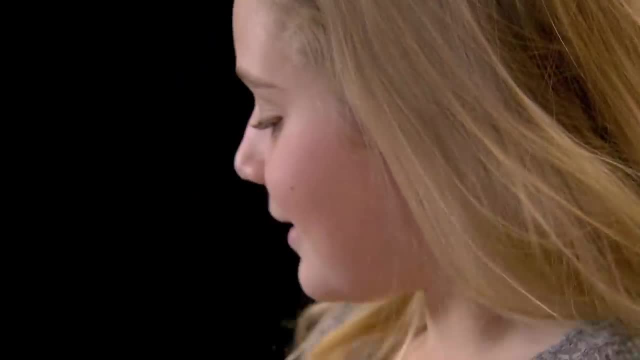 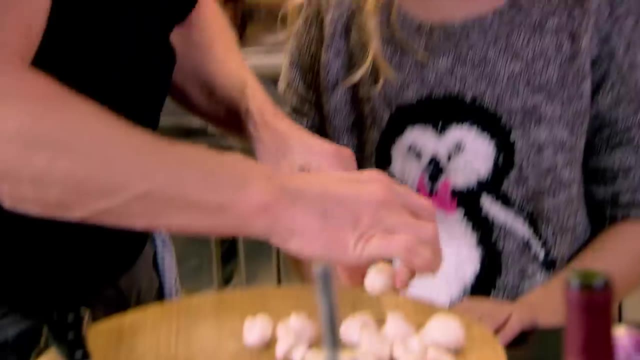 You love hot pot And you love sausages. right Yeah, What do you enjoy most about sausages? Um, I just love having them with the baked beans, sometimes With baked beans. sometimes These are little button mushrooms. OK, you just take them into there like that. 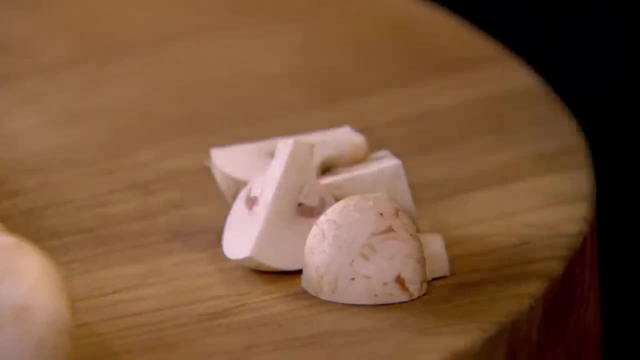 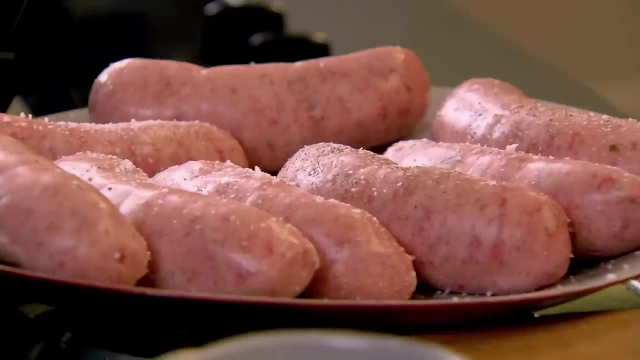 And keep them whole And cut them into quarters, please. Now, the important thing about cooking sausages is they need a bit of colour, right? No colour, No flavour. Exactly, Get the pan nice and hot. How was school today? 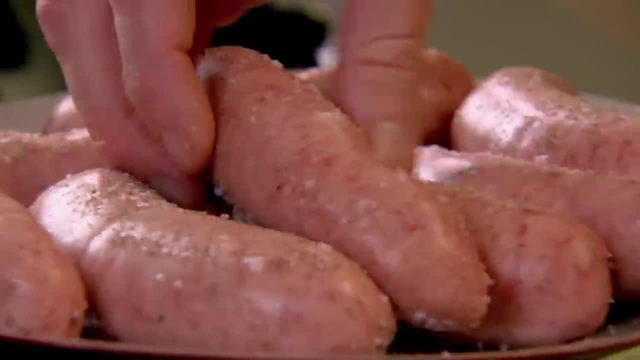 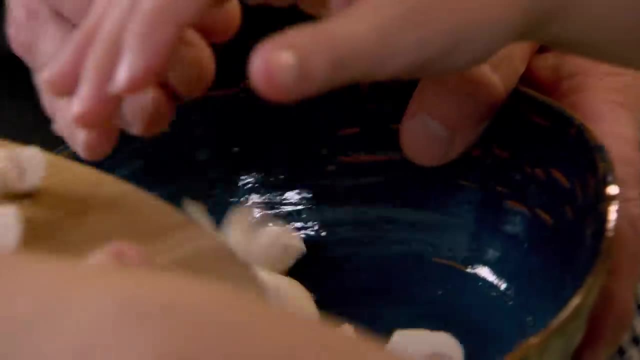 School was good, thanks. We got to go out and mix. no more Sausages in Sausages in. OK, Butter mushrooms in there, please, my darling. Ah, Ah, See, Now I want you to watch your fingers. 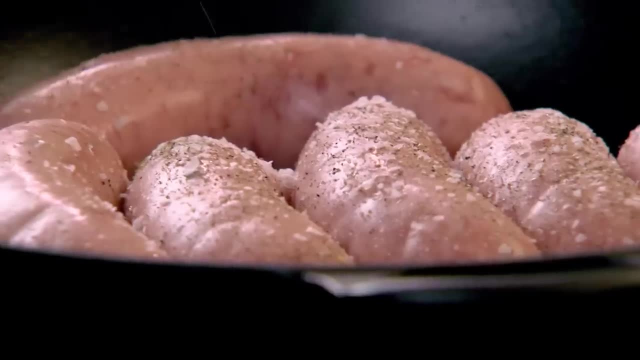 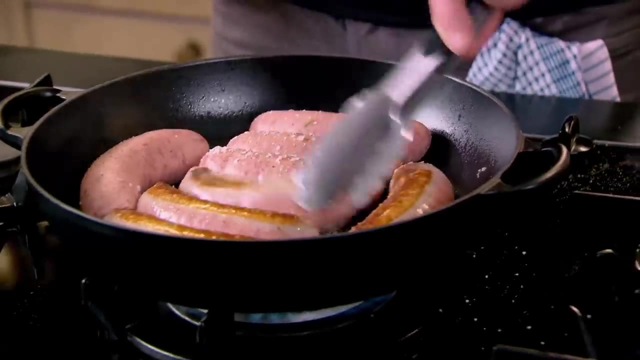 but you know how to slice onions right. Definitely Off you go darling. Now Sausages are getting lots of colour, cos this is going to cook slowly and it's sort of Daddy's version of the kind of hot pot. 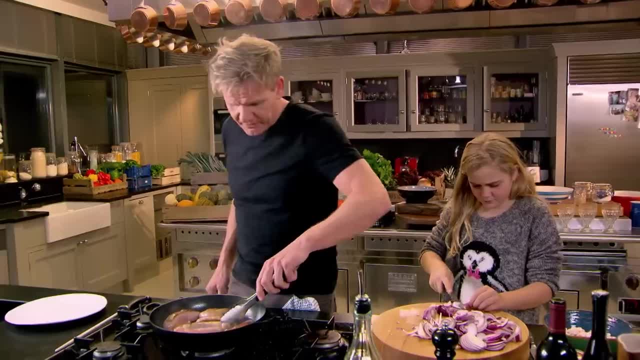 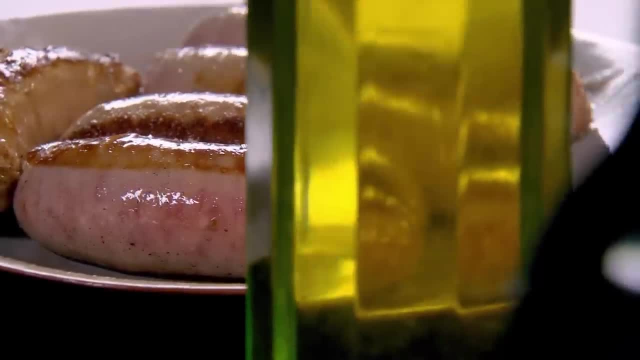 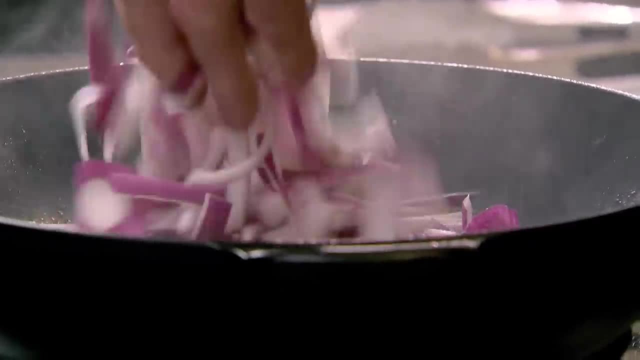 You know the one Nanny used to make for me. Yeah, Once you've got the colour on them, you take them out to rest. OK, A little knob of butter. OK, into the pan. Now it looks like a lot of onions, right. 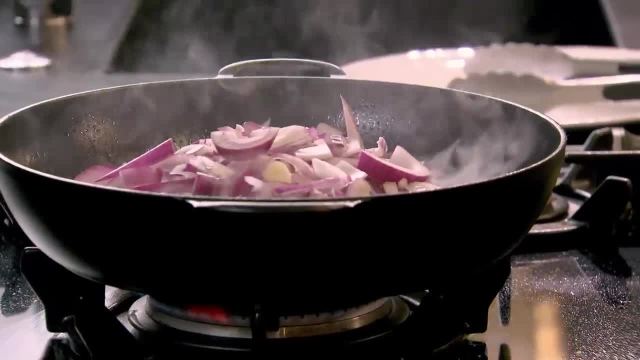 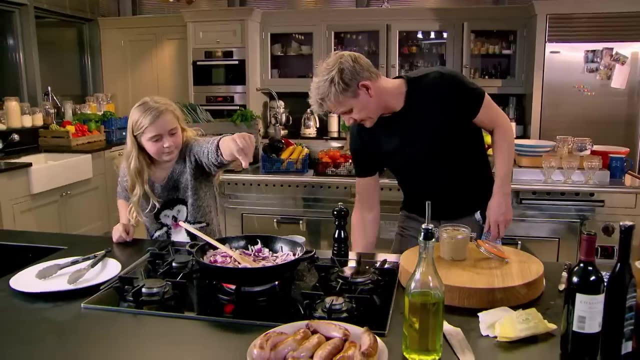 Yeah, As they start sweating down they caramelise, so that will go down by half. Give that a little fry. OK, Salt in. I want you to put a nice tablespoon of brown sugar in there. That gets them really nice and dark. 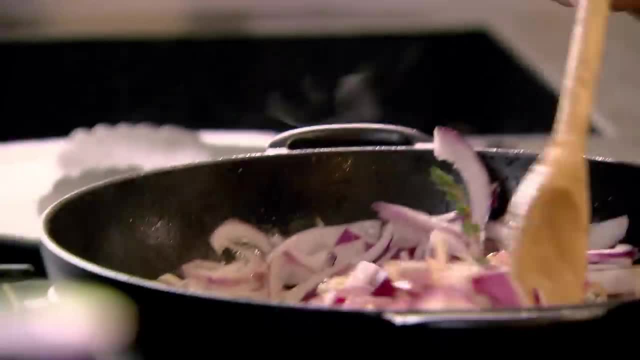 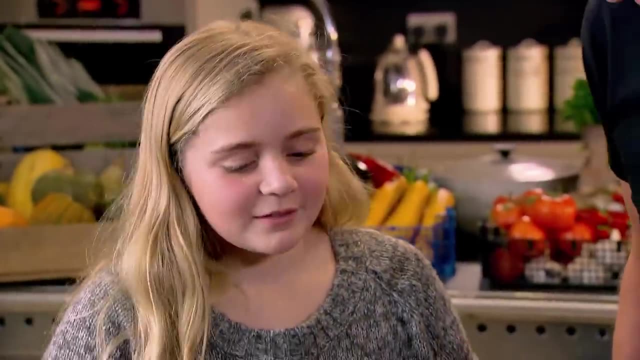 Now get your thyme in. Pick off all the little buds That will get the onions packed with flavour. Mmm, That smells nice Mushrooms in. Give them a nice little stir. Did you like to help Nanny make your hot pot? 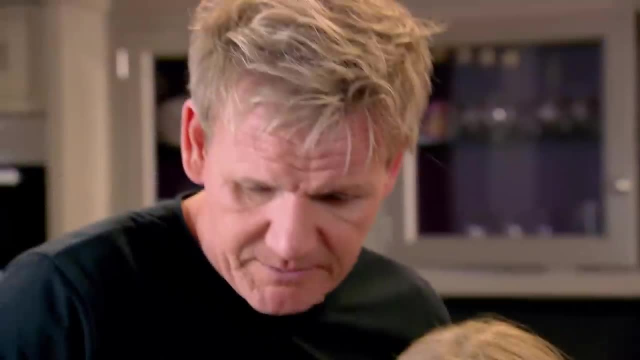 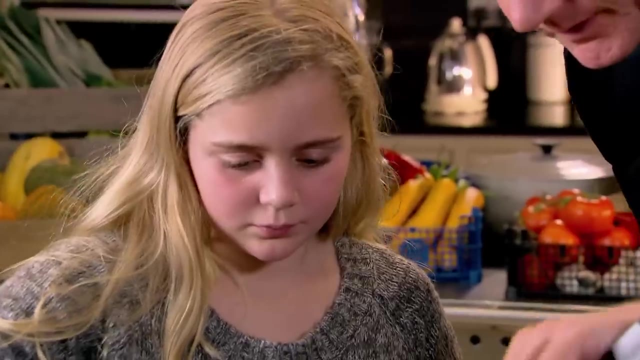 when she made them for you. I used to always help Nanny make the hot pot, Always. Now my mum would never have used this, but A's balsamic vinegar brings out the flavour of the onions. Right now. look at our onions. 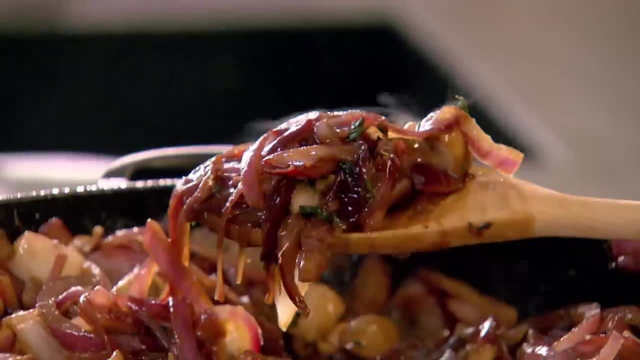 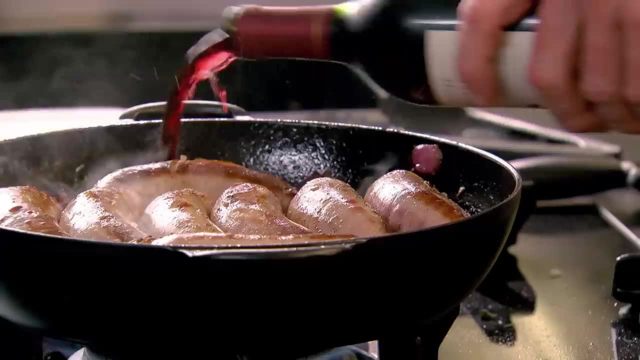 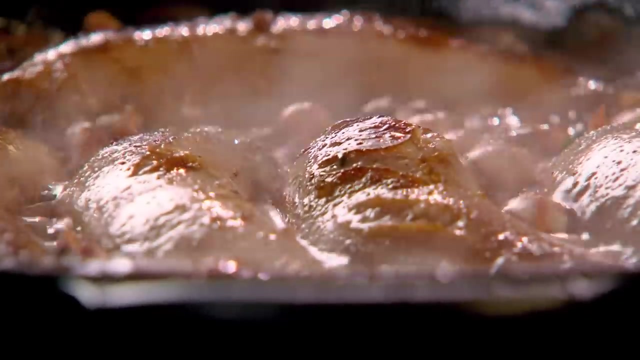 Look beautifully caramelised The vinegar's. given that nice sort of gloss, I'm going to put my sausages back in here now. From there, some red wine. Red wine in. Got the flavour underneath there going into the sausages now. 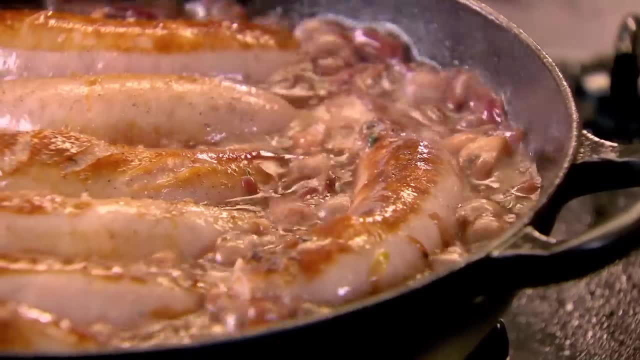 The sausage is going to release all that flavour inside as well. Look at the colour of that And the smell. And it's still not cooked yet Up to the boil. Really important to boil it here, cos it won't boil in the oven. 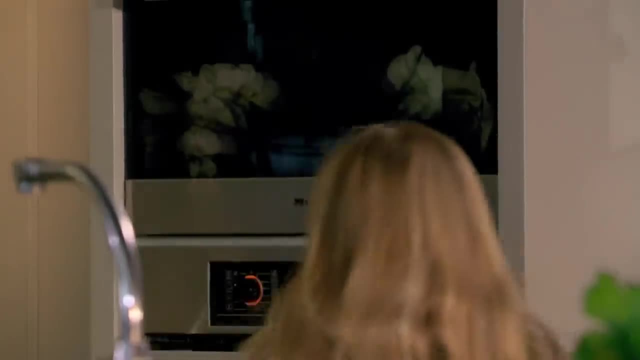 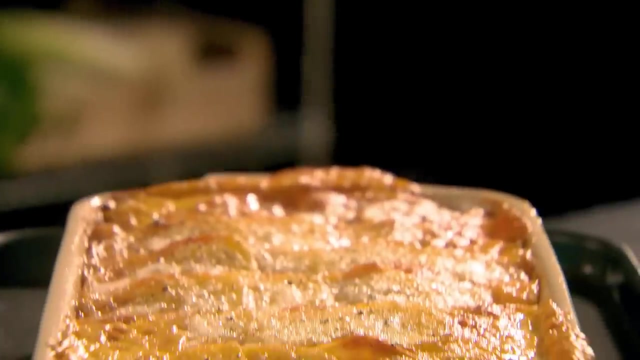 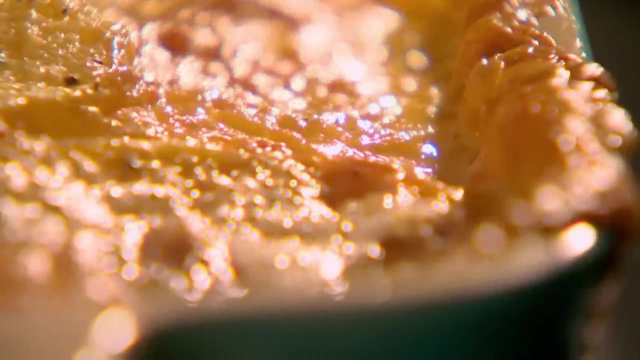 170 in the oven, Literally 18 to 20 minutes In. she goes Nice To go with my hot pot: rich golden creamy potato gratin. It's a true comfort food classic, and I'm adding a delicious twist. 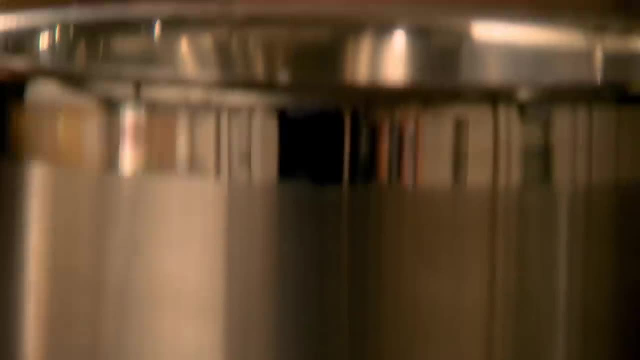 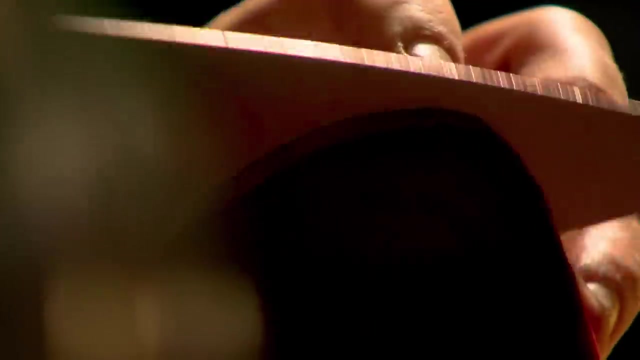 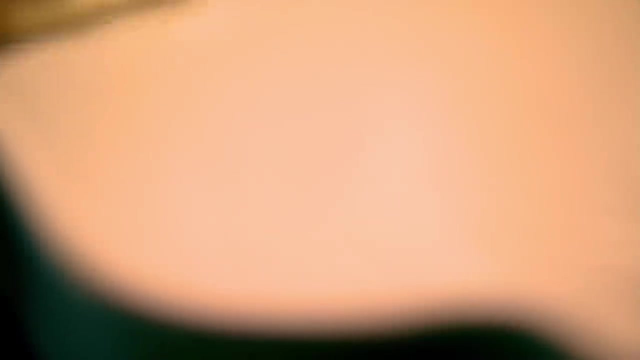 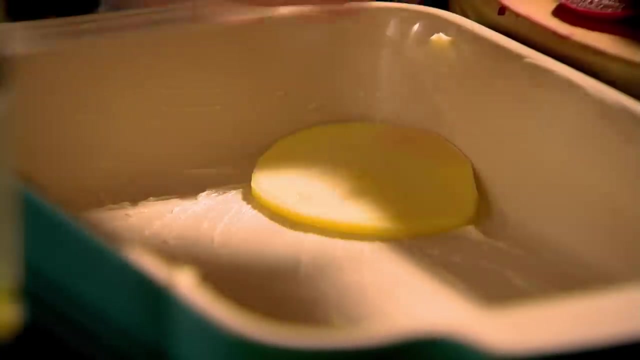 Beetroot. Start by gently heating double cream. Then peel and thinly slice potatoes and cook beetroot. Next rub garlic around the edge of your dish to thoroughly season with their glorious flavour. Then grease with a good layer of butter, Arrange alternate layers of potato. 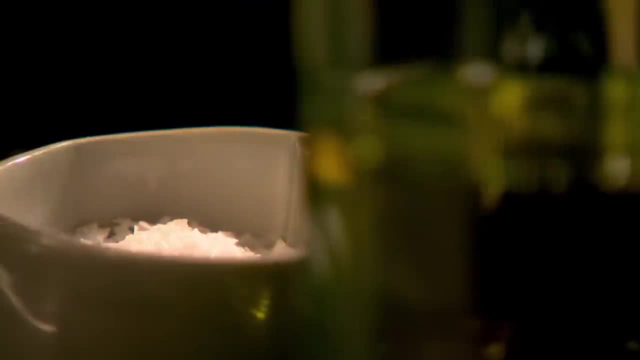 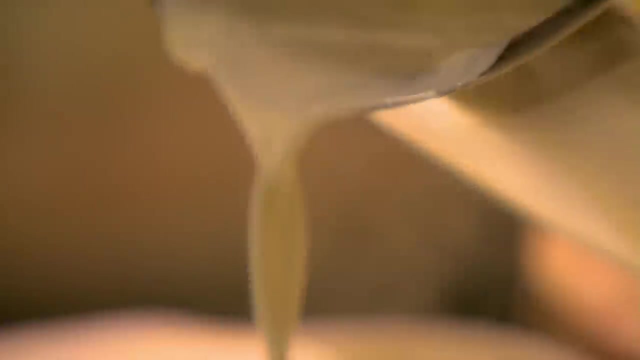 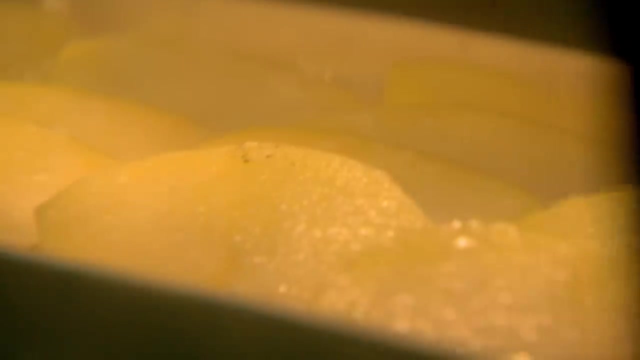 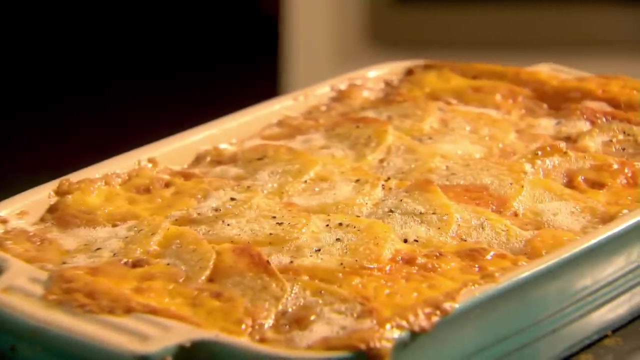 and beetroot seasoning. in between, End with a neat layer of potatoes and pour the hot cream over the top. Bake in a preheated oven for an hour or until the potatoes are tender. Potato and beetroot gratin are bubbling beauty of a comfort food dish. 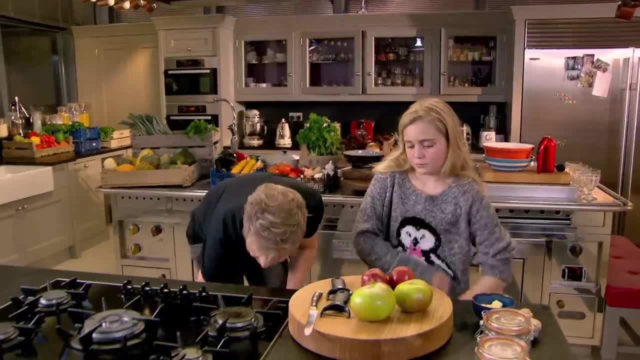 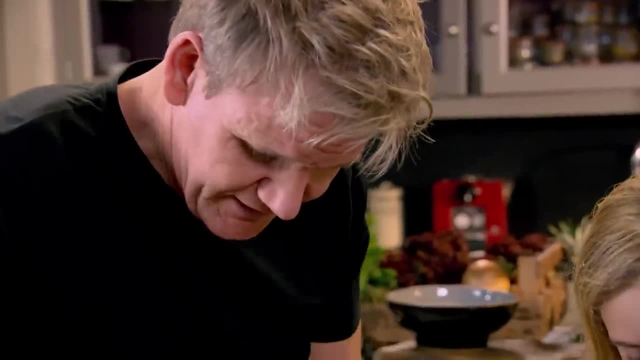 Now for the apple compote. What we need to do first is to get these peeled and sliced. I get my pan on to get nice and hot. Now let me give you a little taste of that. Mmm, it's a bit sour. 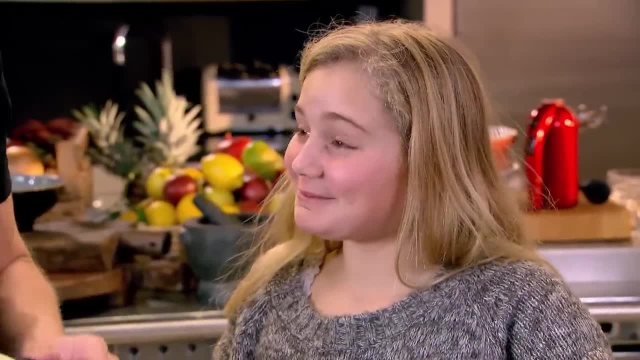 Isn't it? Thanks for the warning. Whoa, So whoa Nearly blew my head off. They're incredibly acidic, okay, and you need to cook them. Those wonderful red apples you've got are called Braeburns. 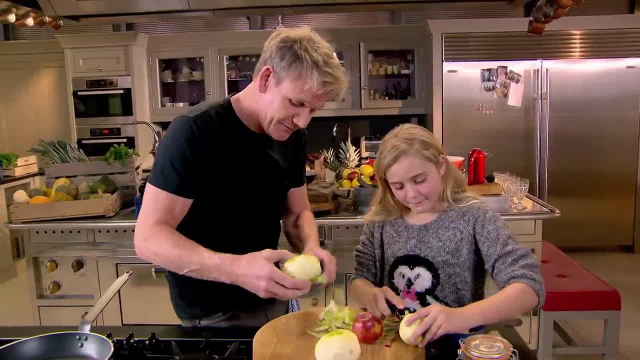 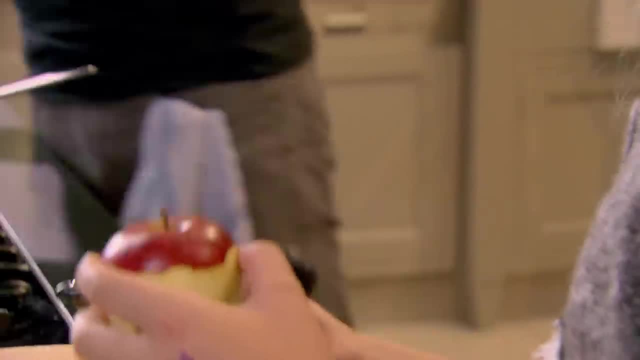 What other apples do you know? Green ones, What are they called? Um, I'm not too sure what the green ones are called. Another word for your nan Grandma's- No, Grandma's Grandma's, Grandma's Grandma's. 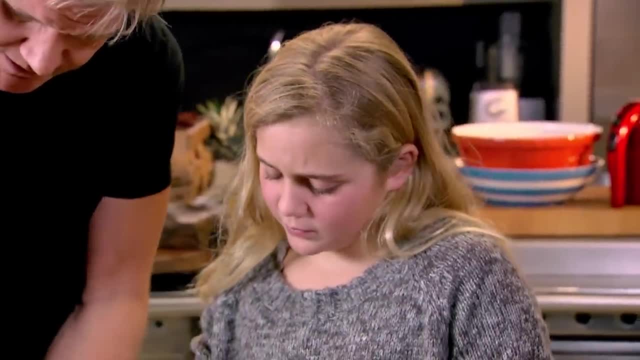 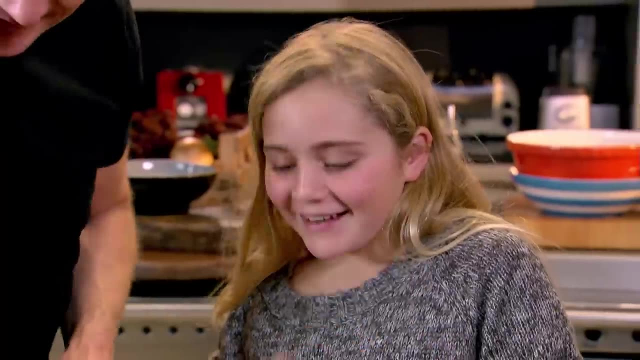 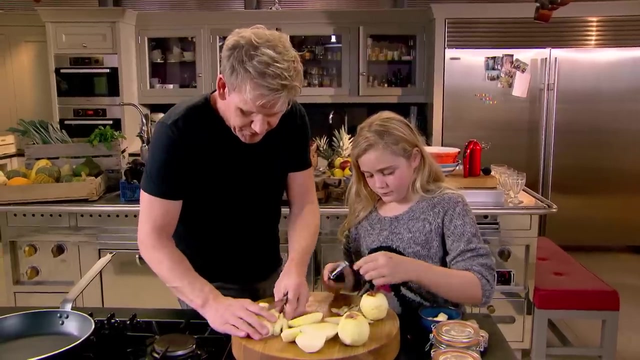 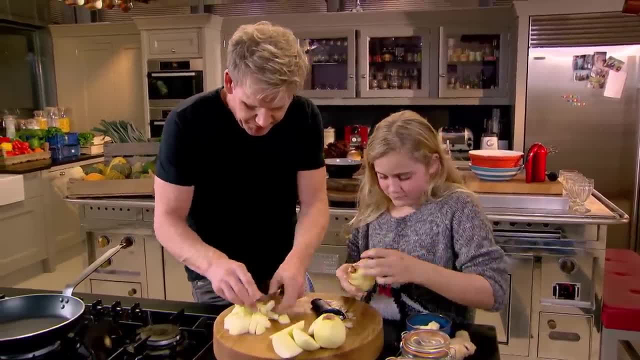 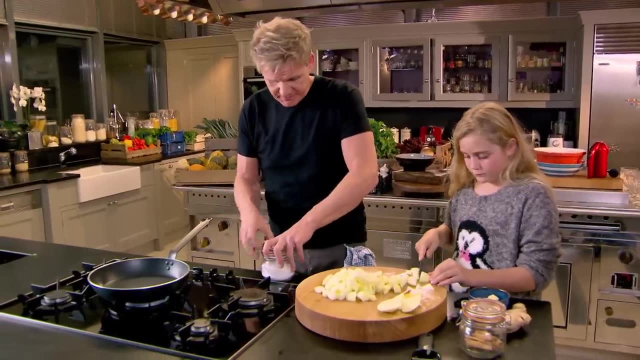 and the eating apples together. I love the combination of the tartness from the Bramley cooking apple with the sweetness of the Braeburn. Get the pan nice and hot and sprinkle the bottom of the pan with caster sugar. Three or four nice slices of fresh ginger. 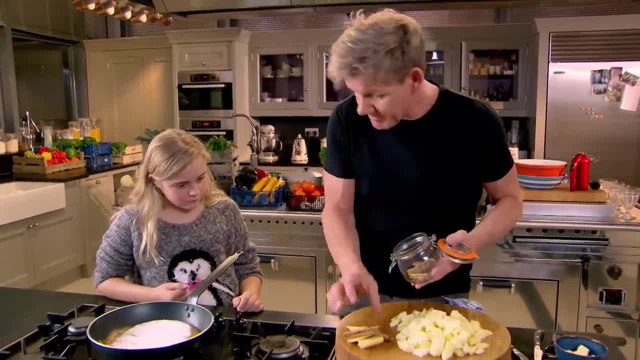 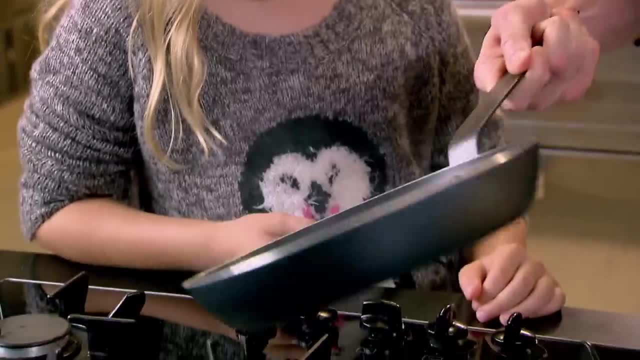 And three little cinnamon sticks. I want you to remember that, because we're going to look for them. OK, Because once we've used them and they've worked their magic, I need to pull them out. See all the sugar dissolving Definitely. 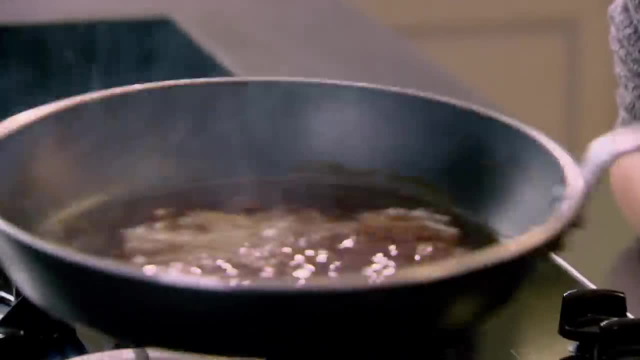 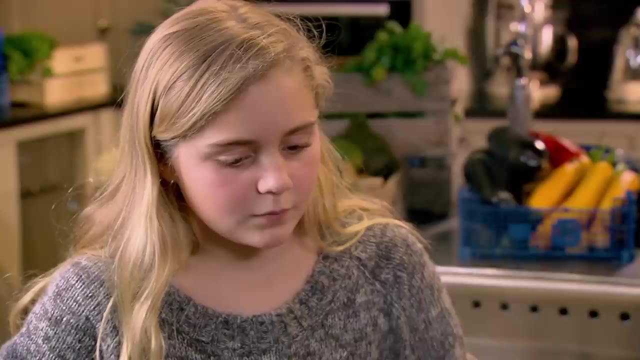 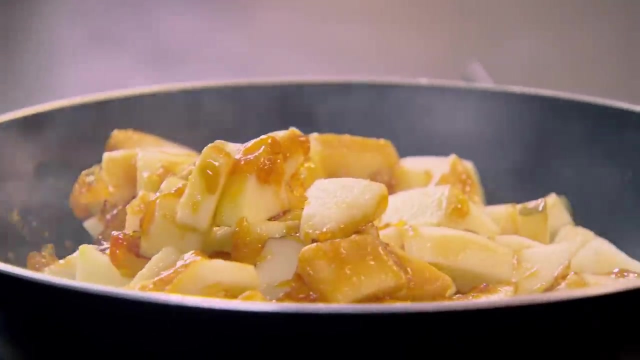 Now we just let that go a little bit darker, OK, And then we place our apples in. It's very quick, Doesn't it? Give that a nice little toss, OK, Nice golden colour Cinnamon in ginger in. 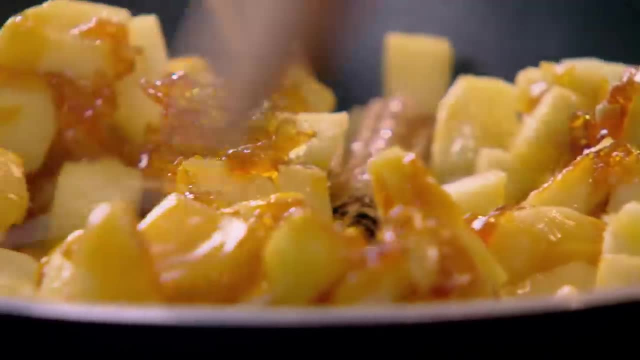 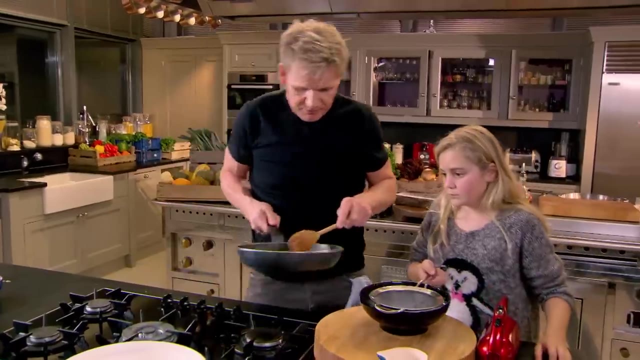 So we're cooking down the apples Butter in Gently cook until the apples soften, then take off the heat And we go into there. What's that coming out, Dad? So that is a little bit of the puree. 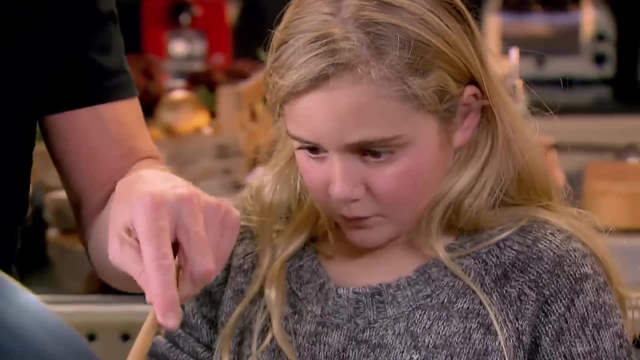 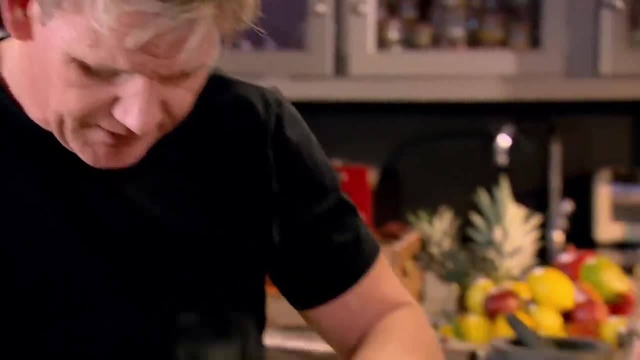 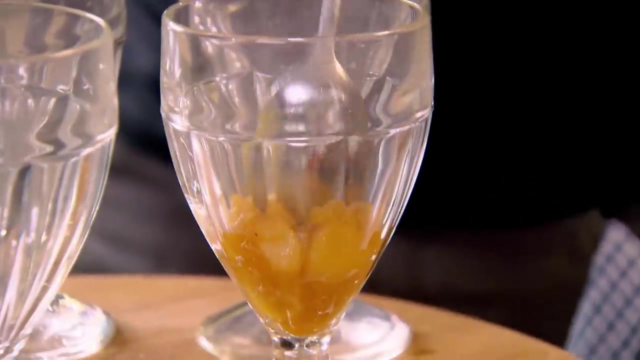 I'll show you how to do that in a minute. How many ginger? Four, Four ginger And three cinnamon. Three cinnamon Out with the cinnamon And the ginger. I've got two gingers And the ginger And we take a spoon of apples and put them in the bottom. 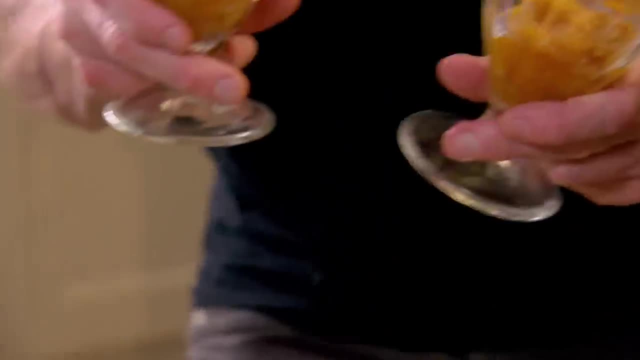 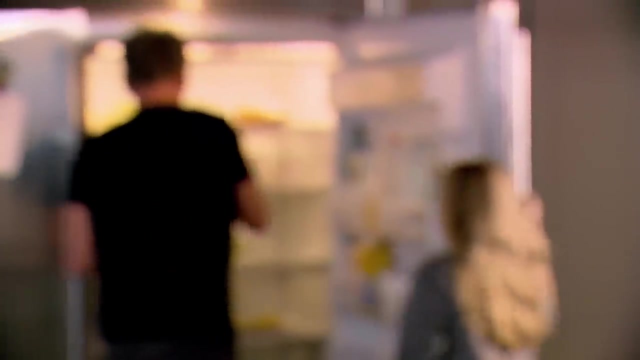 It smells so nice. How nice does that look? See the colour of the apples, Mmm, Let's put these in the fridge to get nice and cold. That's the compote sorted Easy. Now a simple creamy whip to crown the top. 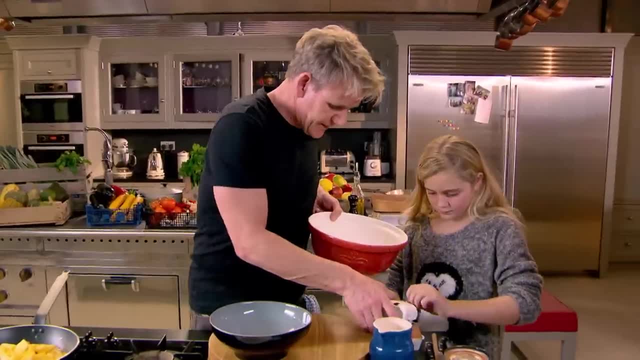 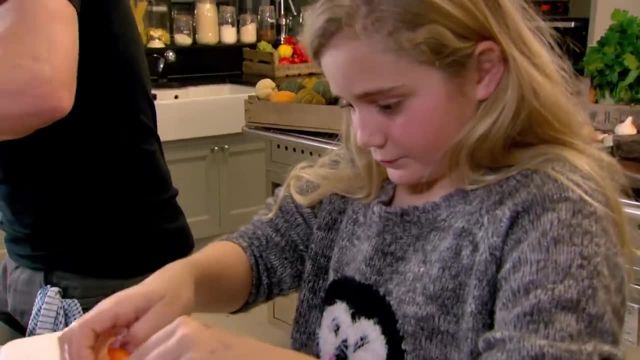 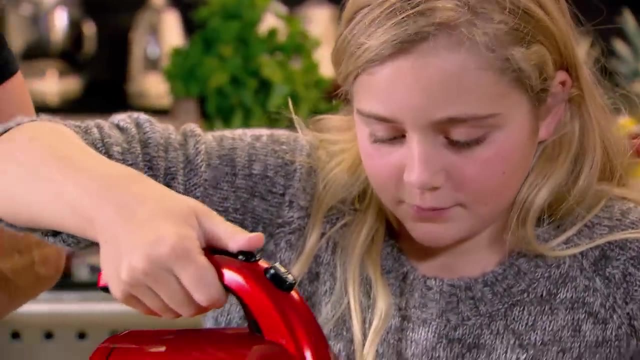 Do you separate the egg whites into? there, for Daddy Right, Egg whites are in, Egg whites are in. You want to separate Off? you go, darling, And I'll sprinkle the sugar in, and then you turn up the speed. Good girl. 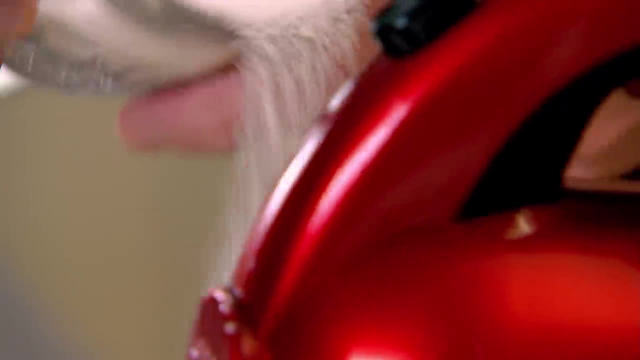 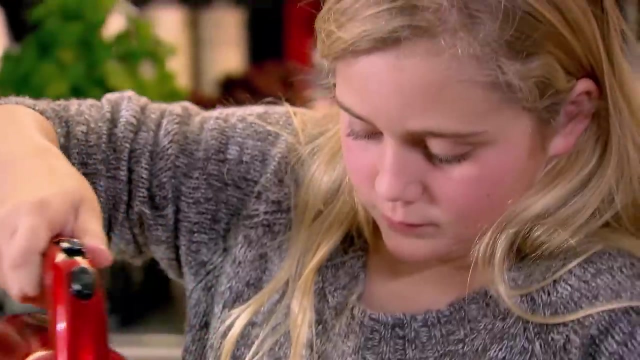 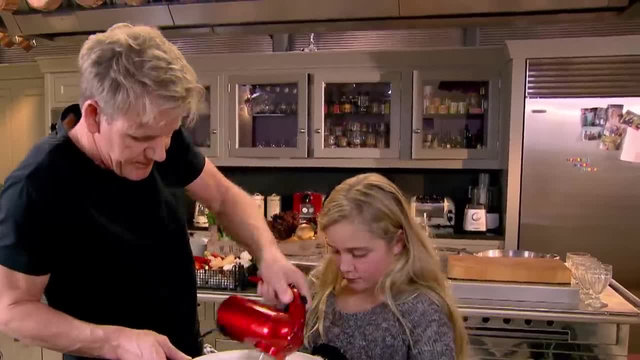 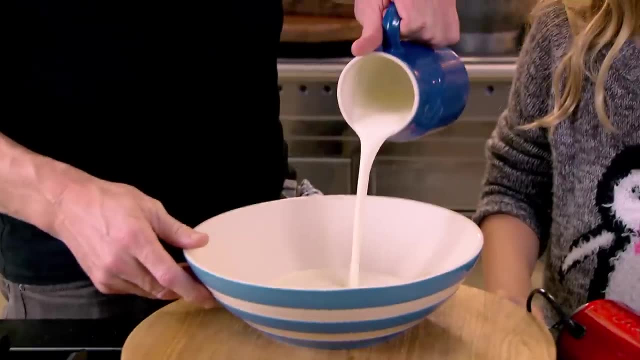 There you go. Now let's see if you've got a really nice stiff peak. So you lift them up Now. that is what I call a nice stiff peak. Well done, Not bad, Not bad. Next, in a separate bowl, whip double cream until stiff. 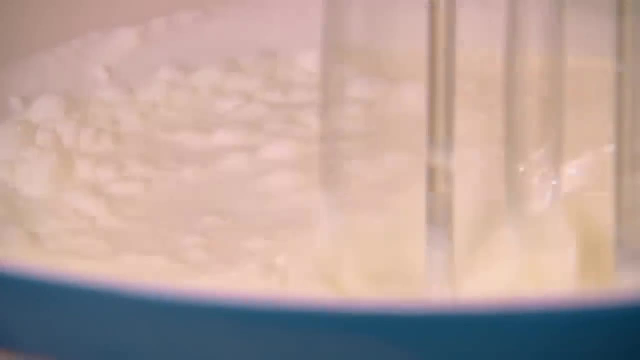 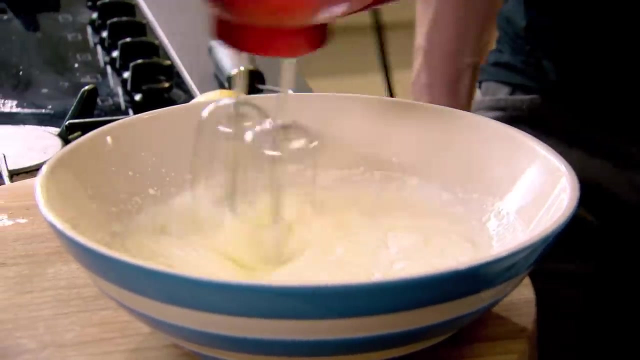 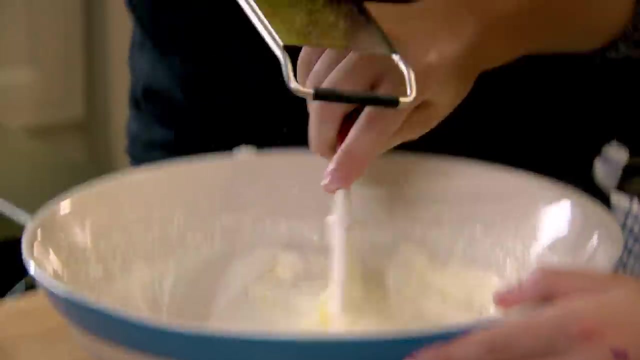 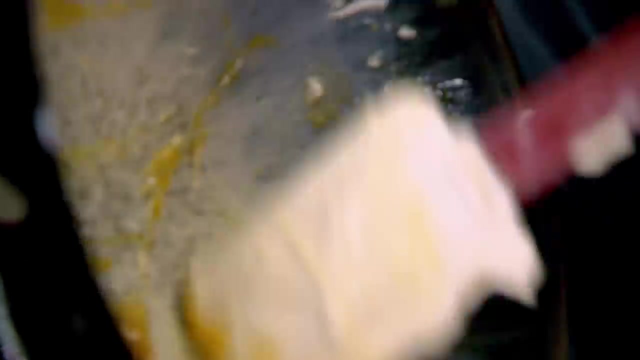 Nice and slowly. So cream whips so much quicker. Yeah, Nice, Is that by hand. Dad, We're going to put some cream in Delicious lemon zest, which will make the cream so much better, Then sweeten it up with leftover caramely compote puree. 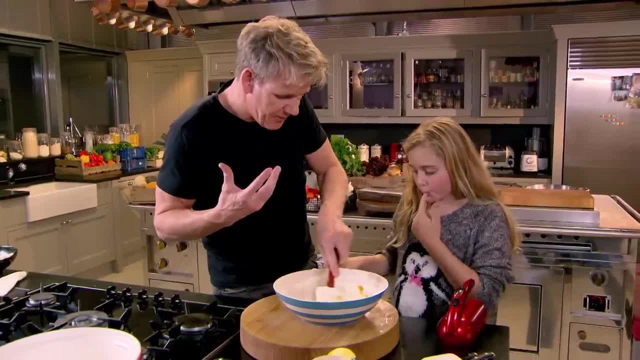 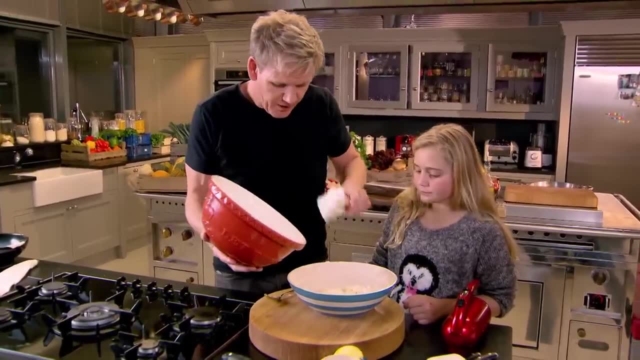 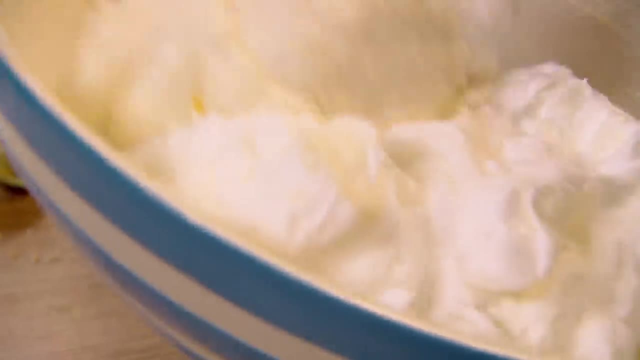 You mix that in nice and carefully, So it's like this apple butterscotch. Now, to make the cream even lighter, fold in those whisked egg whites and sugar Egg whites into the cream. Just nicely fold that in. So bring your glasses back out. 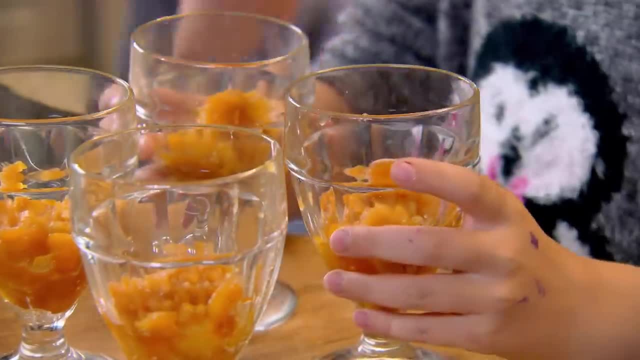 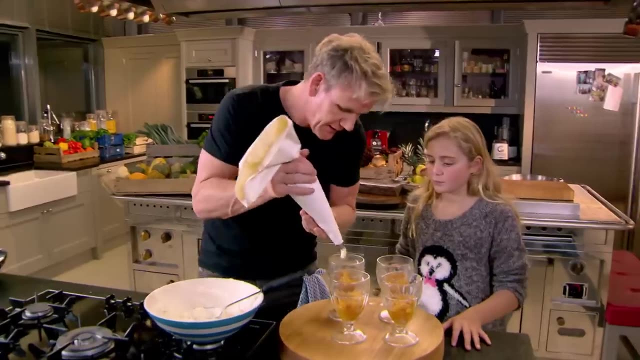 Manage the glasses. Yep, Good girl. Mm Silly, We're on for a treat. Open up the piping bag Now. twist the end Now. you could spoon this in, but I want to just give a nice little lift. 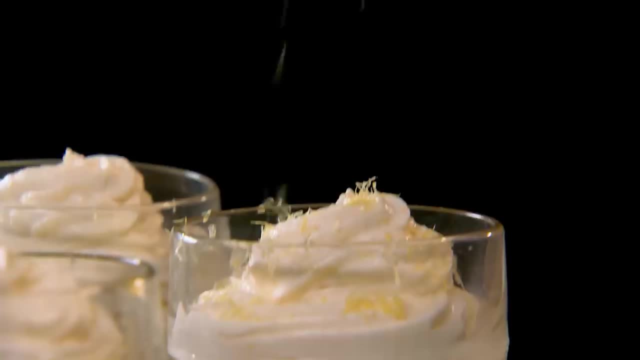 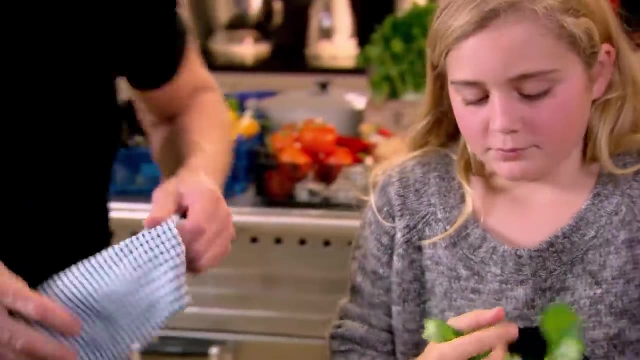 It also gives it a nice pattern. Lemon on top, Back in the fridge. The beetroot and potato gratin- Mm, Isn't that lovely, That's lovely. And the sausages, Ooh, Mm. Flat-leaf parsley. 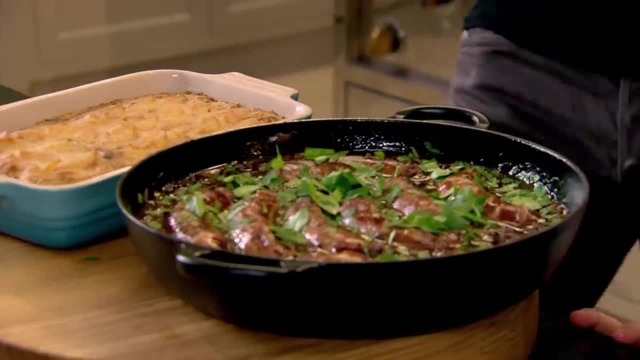 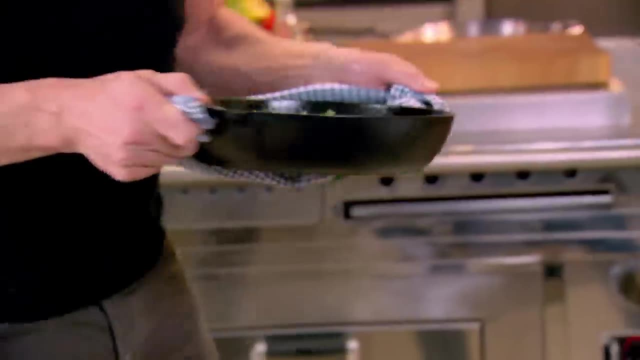 Now look at those two beauties. Mm, It doesn't get any more comforting than that, does it For one of the best hot pots ever. Tilly, that looks amazing. I know, Well done. This is my ultimate comfort food dinner.